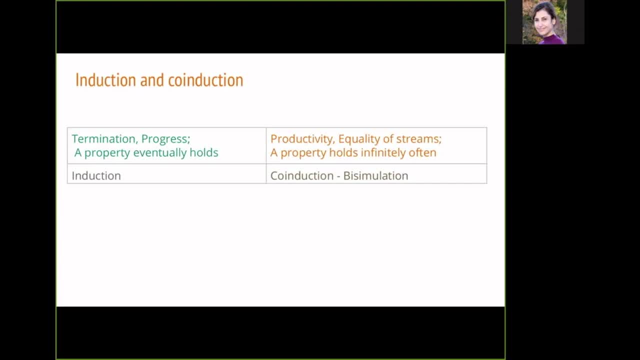 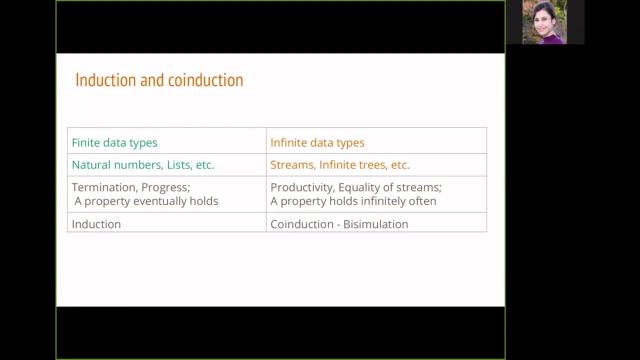 to prove properties that hold infinitely. often, The object of interest in an inductive argument are finite data types, like natural numbers and lists, while in co-induction we are interested in infinite data types like streams or infinite trees. To be more accurate, we need least fixed. 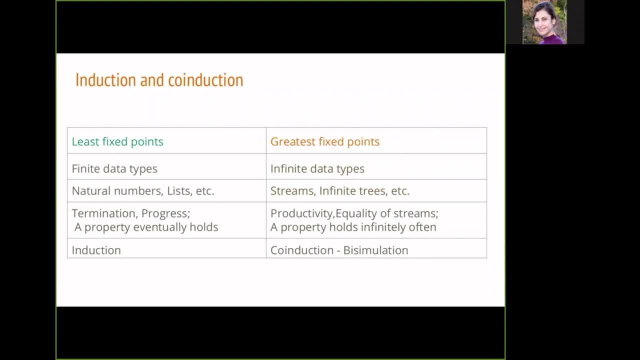 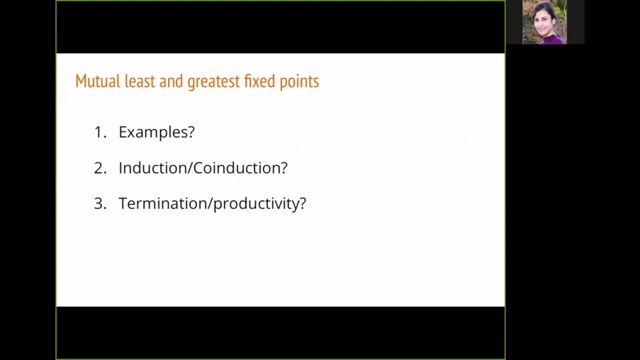 points to apply induction on and greatest fixed point to apply co-induction on. So the main question that we pursue in this talk is that: what everyone should know about co-induction. So the main question that we pursue in this talk is that: what everyone should know about co-induction. 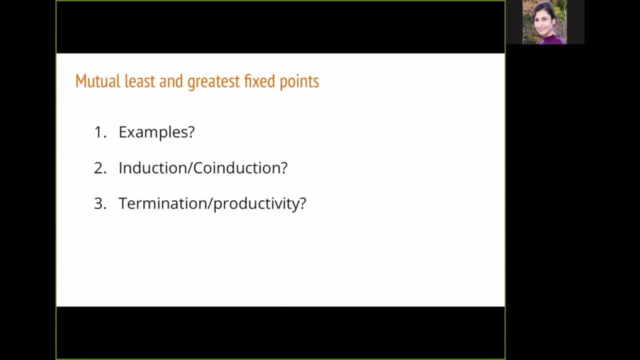 to work with data types defined as mutual least and greatest fixed points. Are there any good examples of these data types? Well, the short answer is yes. An interesting class of examples are the programs that work on mutual least and greatest fixed points, And then which principle? 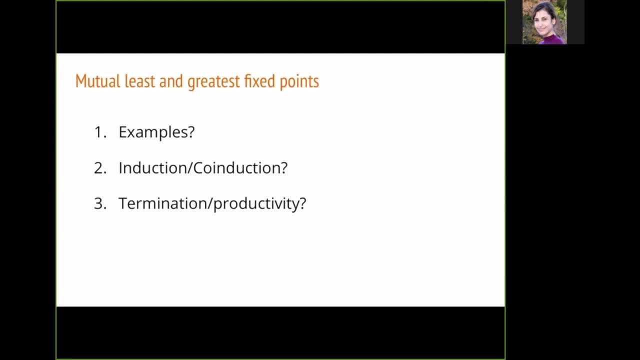 shall we use to prove properties about these programs? The first guess, which is actually correct, is to apply induction and co-induction simultaneously, but we need to be more conscious with mixing these principles. And finally, if with induction we can prove termination and with 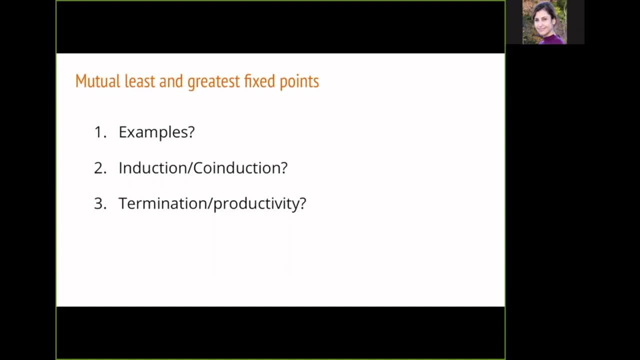 co-induction we can prove productivity. what property can we prove with the simultaneous induction and co-induction? We want to analyze the answer of these questions, but first let's review some previous works. Well, we are all familiar with induction principle and 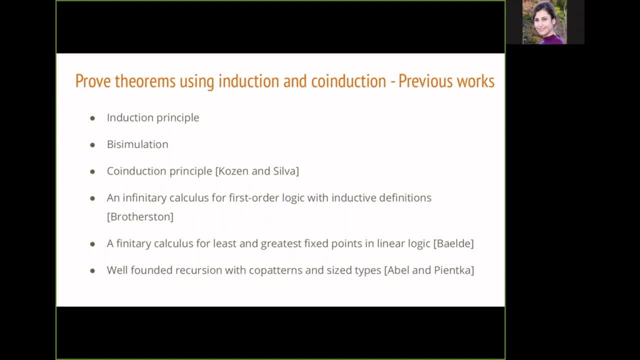 by simulation, And Kozan and Silva presented a co-induction principle in their 2017 paper. Now you can find a pointer to it in the references. We also adopted a couple of their examples in this talk and in our paper. In his 2005 paper, Broderson introduced a first order calculus that allows 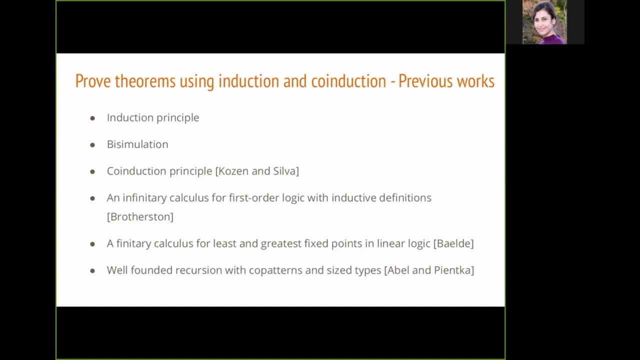 for circularity. The circular edges in his work are representing inductive steps and he introduced a validity condition to ensure that these inductive steps are good. In this talk, we follow his approach, but we want to enrich our system with co-inductive cycles as well. 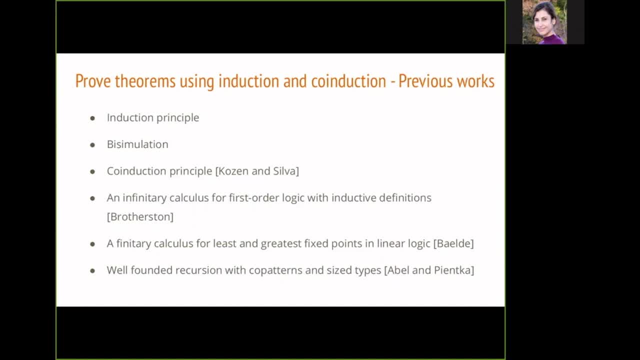 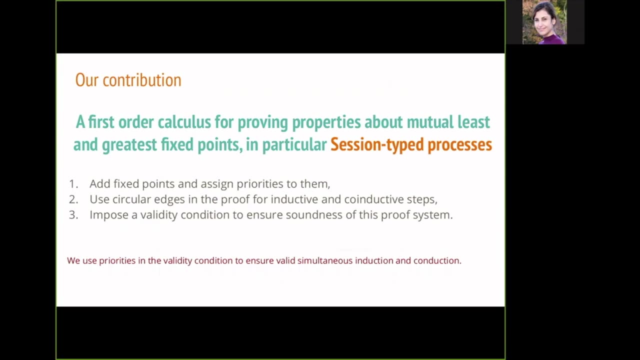 There are some other proof-theoretic approaches to mix induction and co-induction, For example the finitary calculus introduced by Balde and Saez-Saez by Abel. So far we have established that our goal is to introduce a first order calculus for linear logic. 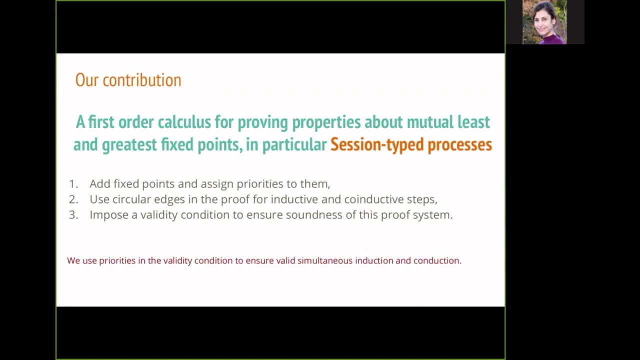 and reach the least and greatest fixed points. Following the approach of Broderson, we allow circularities in our system and our circular edges correspond to co-inductive and inductive steps And of course we need a validity condition to make sure that these steps are good. 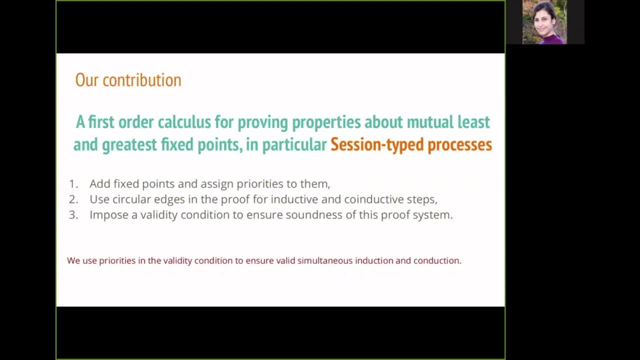 I'm not going to explain our validity condition in detail. If you're interested, you can take a look at our archive papers. but I want to point out that for our validity condition, we need to assign priorities to least and greatest fixed points in our system. You can understand these priorities. 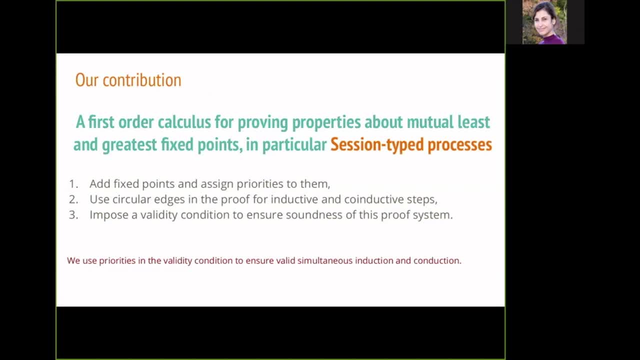 as the order in which you solve asset of least and greatest fixed point equations, And also for more information on this you can take a look at Fortier and Sando Canola's paper. I will point you to that in the references too. 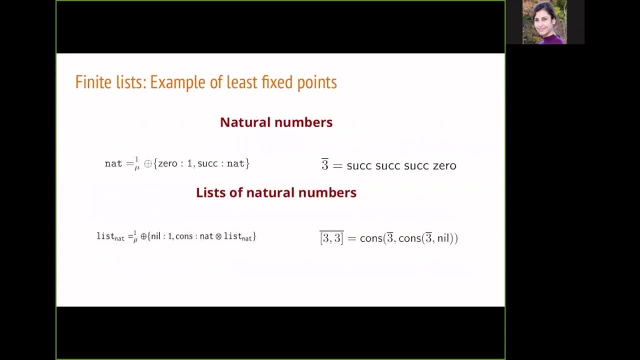 Now let's take a look at an example. We have the natural numbers as the least fixed point of zero, of type one or successor of type natural numbers, And the list of natural numbers is the least fixed point of an empty list, which we call the null, or it comes of a natural number with a list. 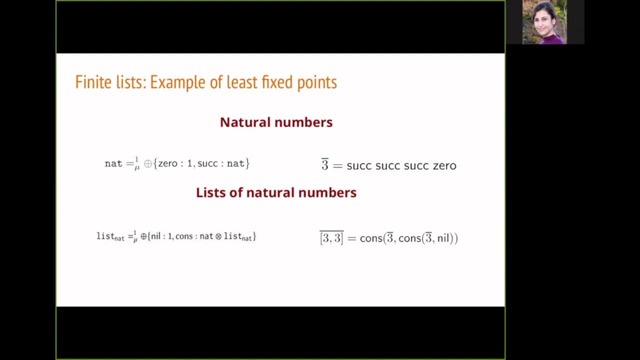 continuation. So mu in the subscripts of these definitions stands for least fixed point And the one in the superscript is the priority assigned to these types. Of course, since we don't have any greatest fixed points in this signature, the priorities are not important. 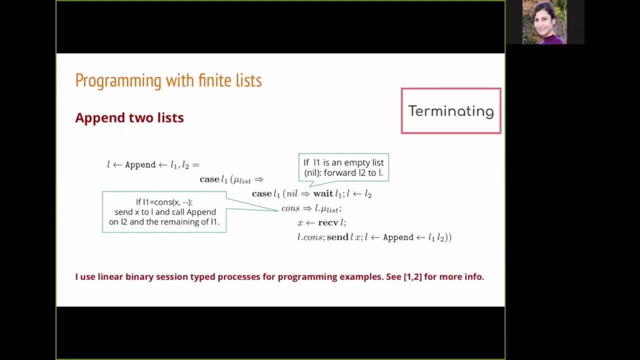 Now let's look at a programming example. Most of the programs in this talk are written in the context of session type processes. I will give you the high level information of them, but if you want to familiarize yourselves better with their syntax, you can take a look at Frank's lecture. 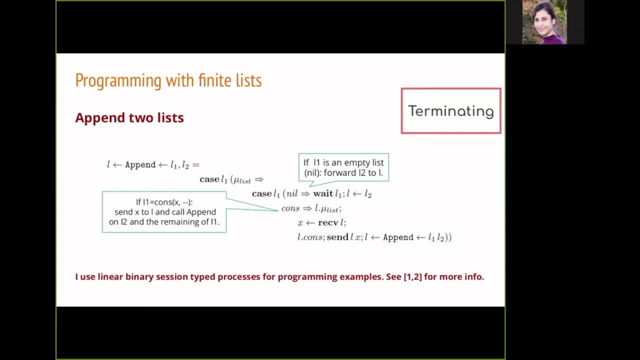 notes that are going to put a point of that in the references. So here's the code for append: It receives two lists- L1 and L2, as it resources and append them in a new list L The way it does. it is the first case on the list L1, this case L1 here. 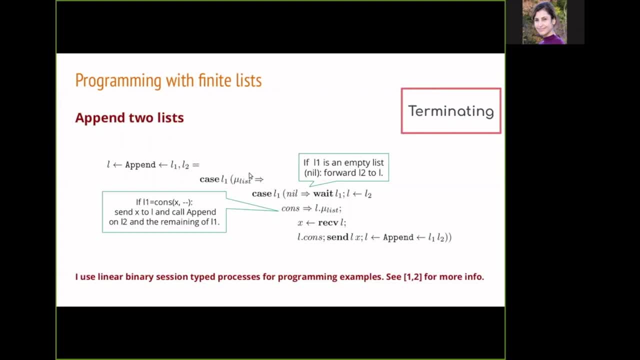 Unfold the definition of list using this new list and then it will look inside the structure of the list. If it is an empty list for null, all we need to do is to forward L2 to L. If it is a cons of some element x and some continuation L1 prime, we send x to L and call append recursively. 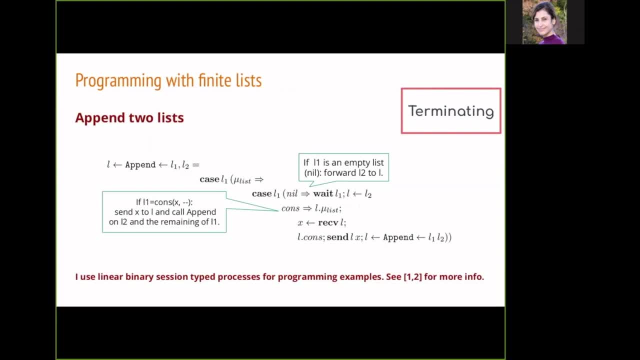 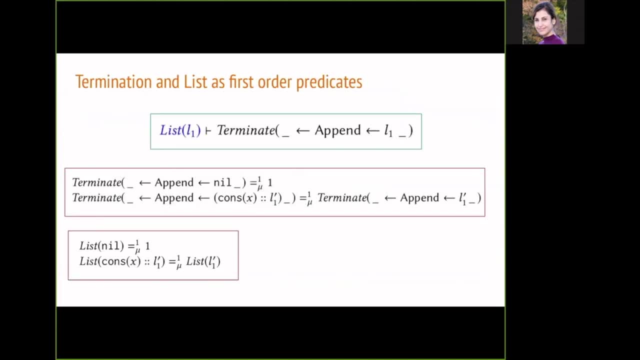 on L1, prime and L2.. I think we all agree that this program is terminating. Now we want to be clear that this is actually the case. We define the predicate terminate and we define it exactly on this program append and we actually use pattern matching to define it. 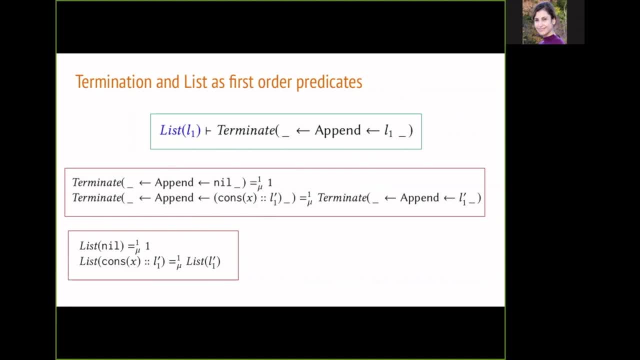 here, but you can take a look at its extended definition in our archive paper. So if the first argument of append is null, then it means that we know that the program terminates. so we just put it equal to type 1.. If the first argument is cons of x and some L1 prime. 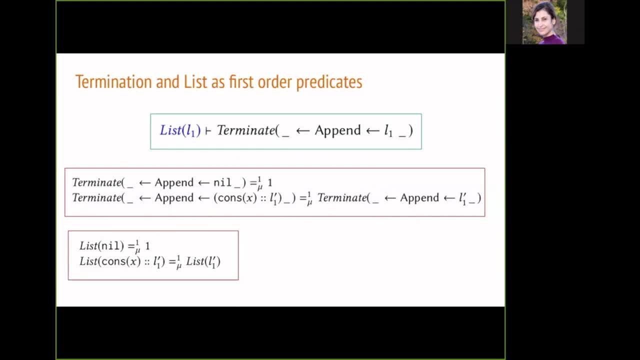 it will terminate only if append terminates on L1 prime. So, as you see, termination of append. for termination of append you only need to have information of the first argument. That is why I put these underscores for the other arguments, because they're not needed in the termination. 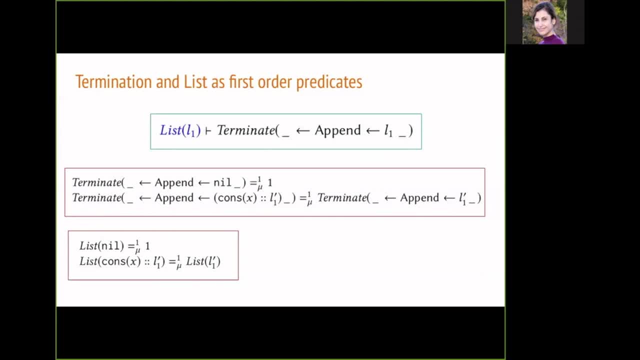 Okay, so similarly, I defined predicate list, where if a list is equal to null, then we know that it is a list, so it's just one, And if it is cons of some element and L1 prime, we only need to know that L1 prime is actually a list. 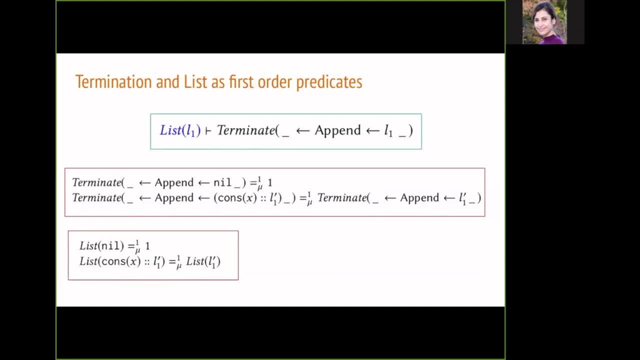 Okay. So, as you may have noticed, variety is first-order predicates with a very similar side to the definition of list and natural numbers. A couple of slides before mew again stands for least fixed points and superscript 1 is their priorities. 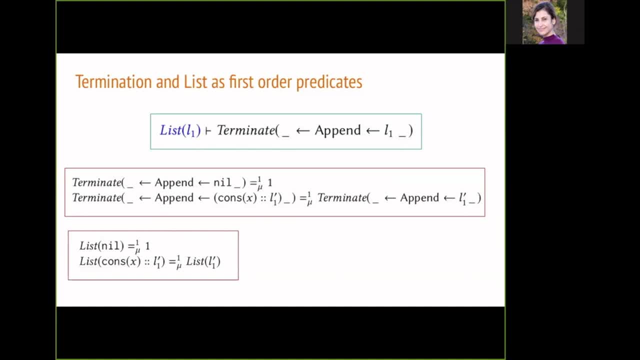 However, here I want to emphasize on the subtle difference between them. Variety are session type programs based on the propositional types and in a meta circular way. we prove properties about these programs using an echo of the model and we can show it in a better way. So we can see that each type of program contains the same level of division and every time that we type one, we get the same number of values. and we can see that every time that we type one, we get the same number of values. 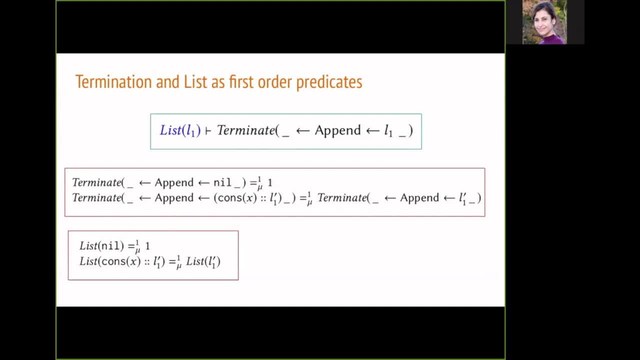 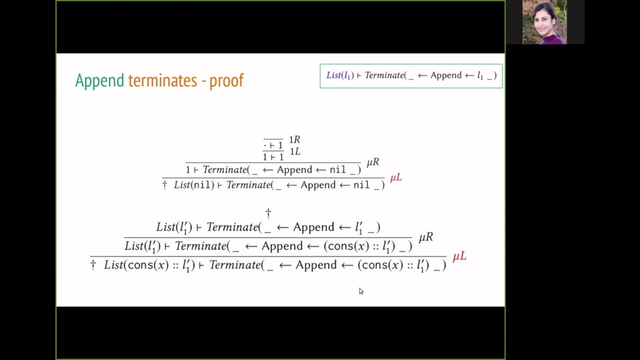 extension of the same language to the first order terms. okay, so now we want to prove this judgment up here, saying that if L is a list, then we can pass it to append as the first argument and be sure that it terminates. okay, so here's the proof. and this is actually a derivation and you can see that this is a recursive. 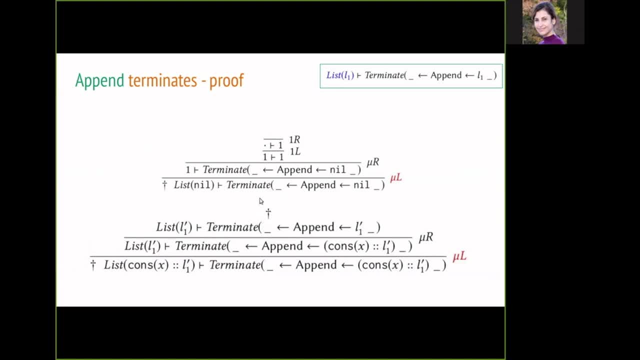 call here. so judgment dagger calls itself, and we know that this derivation is a proof, because this new left occurs here in the circular, in just in this circle. so the validity of this recursive call is ensured by the new left rule that breaks down the definition of a list. 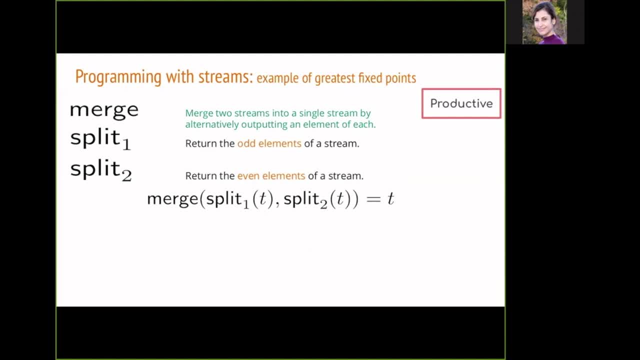 okay, good, now let's take a look at another program performing on greatest fixed points. we have three productive operators: merge, split one and split two. merge simply convert two streams into one by alternatively outputting an element of pitch. split one: return the odd elements of a stream and split two. 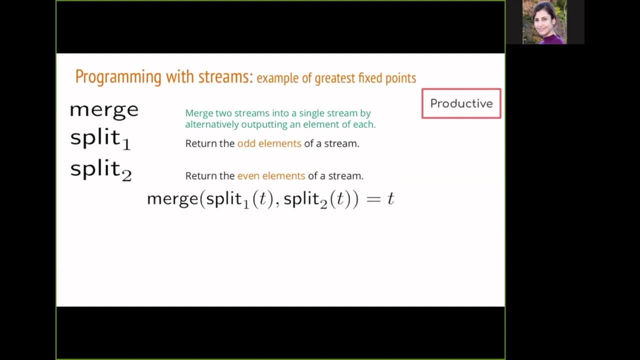 return the even elements. we want to show that these operations are inverses, meaning that if a split, so let's say that this is a stream T, we split T with a split one and a split two into two streams, and then we merge them together again and we build T. so we want. 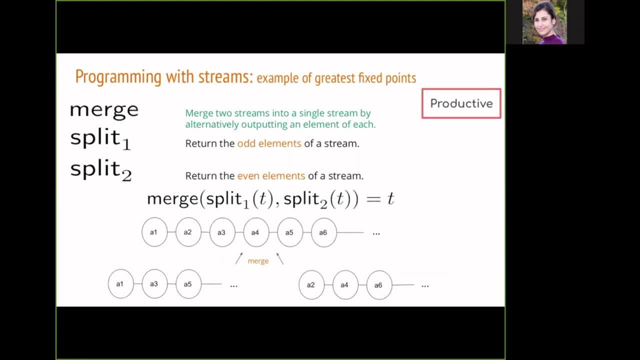 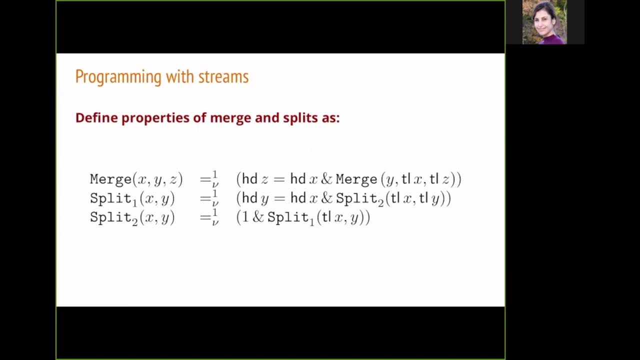 to show that this is actually the case. to do that, we first define three properties for these operations: merge, X, Y, Z says that Z is the result of merging X and Y. it is defined as the greatest fixed point. heads, or first element of Z is head of X and tail of Z is merge of Y and tail of X. 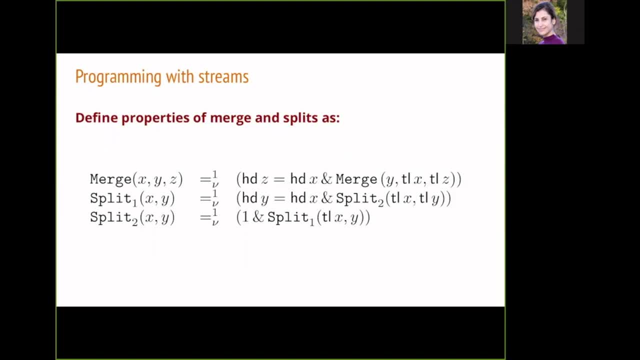 a split one and a split two are defined mutually, again as greatest fixed points. so that is what new stands for. and a split one X- Y means head of Y is head of X and tail of Y is the result of a split two on tail of X, where split two simply means a skip the first. 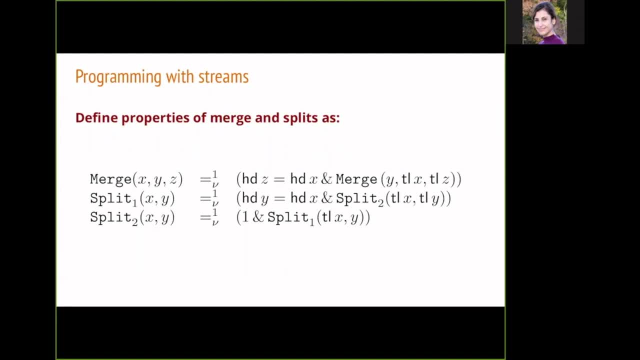 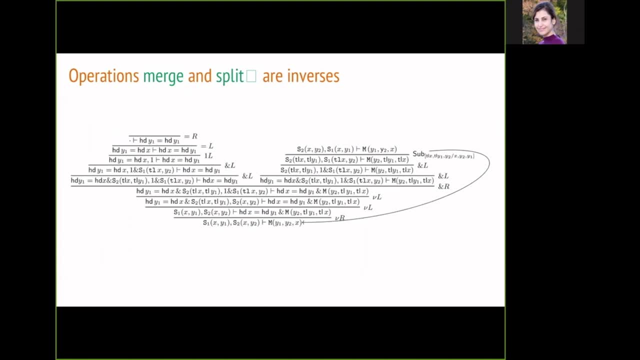 element of X and call a split one on the rest. okay. so here is the circular proof that shows operations merge and split. J are inverses. the circular H-E-A corresponds to a co-inductive step and it is valid because of the very first rule, new right- which ensures that in each cycle we can prove something. 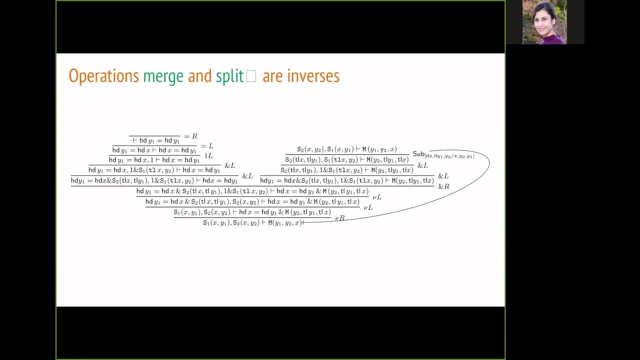 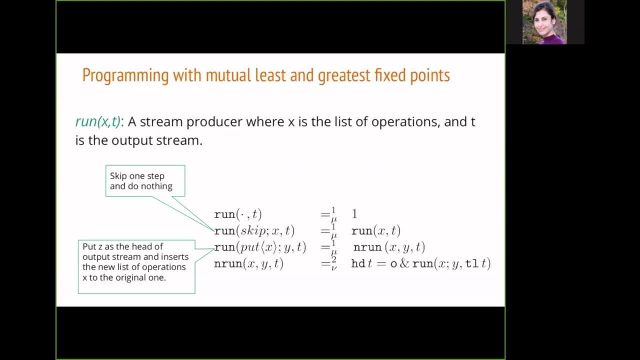 about head of the resulting stream. okay, so, as for the next example, we can look at a more interesting one, which is run XT. this is a string reducer where X is a list of operations and T is the output of the string. if X is empty, it just terminates. if the set up on the list of operations 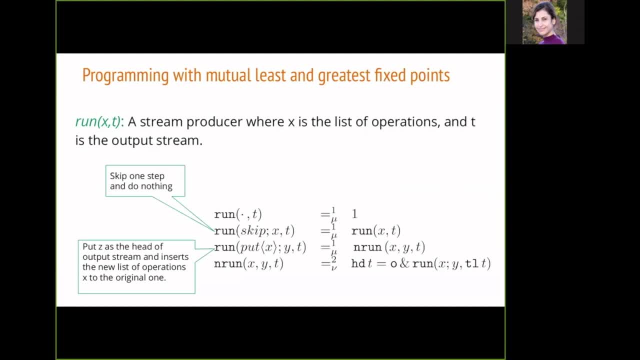 is a skip and then X. it just skips the command and run the rest of commands. if the list of our commands are put X, Y, it will go to a new state which is defined as a greatest fixed points productively, and we call it and run X, Y. 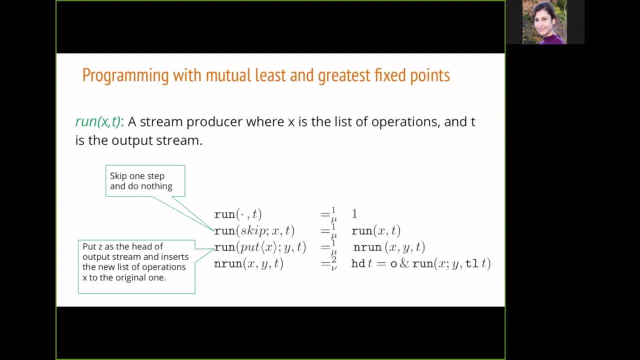 T. it first puts the head of T to be element O and then run commands X and Y sequentially. so you can see that the list of commands grow here. but at least we produce something. the head of T and the priorities are important here because the listing greatest fixed. 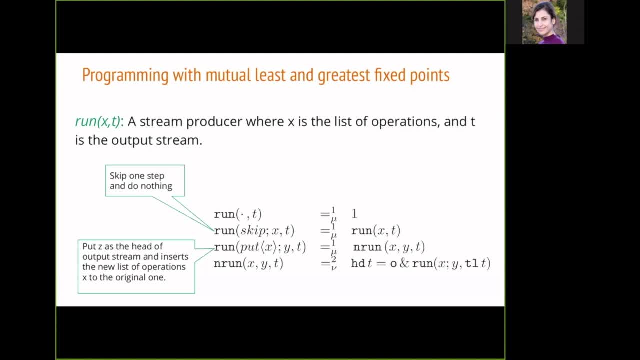 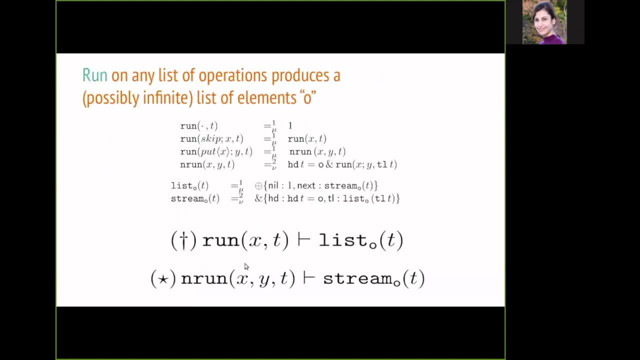 points are mixed together. okay, so we want to prove two judgments simultaneously. these are the judgments that we want to prove. the dagger judgment says that run produces a list of O's and the star judgment states that and LeRoon produces a stream of O's and the definition of List and If stream was. 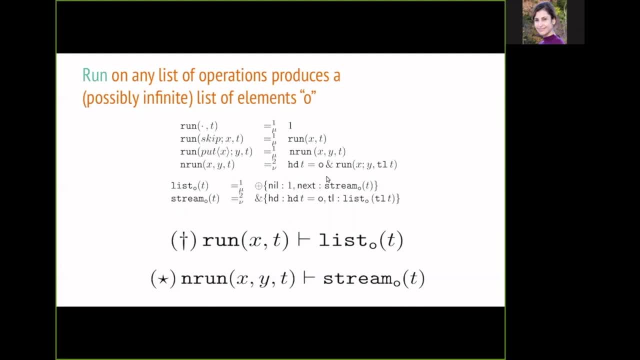 a stream of O's are defined up here mutually, so they're similar to what we've seen for its list and stream, except that they are now mutually defined. so yeah, now that all news have less priority than you. so if news has have priority to and use a priority to. 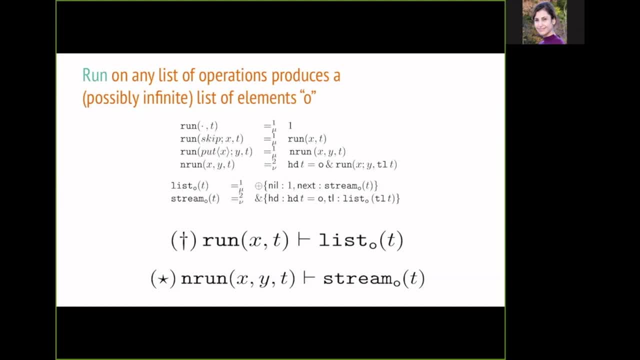 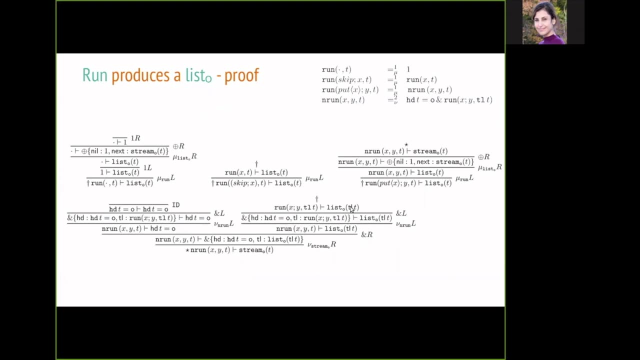 have priority two and news are priority one and related as the news have less priorities um than news. okay, so let's take a look at the proofs of these judgments, uh okay, and, in particular, take a look at this path. so we start from here and then we go up there. 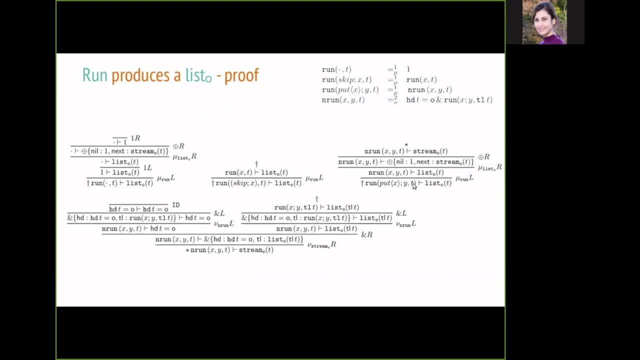 so we first unfold the definition of run- when we have a put, so we get to an end run. and then we unfold the definition of new list and then we choose to um produce a next and stream. and now we- we need to prove this the star judgment which is here- and again we unfold the definition of a stream. 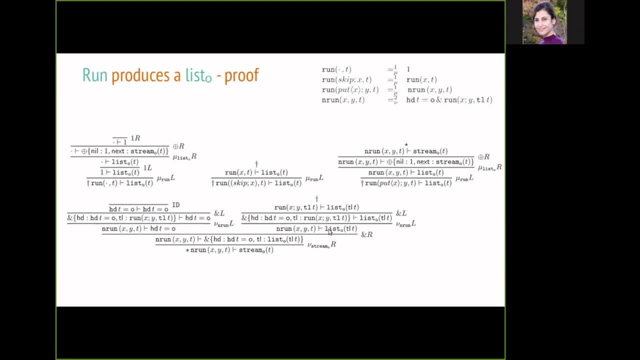 and um, let's say that the, let's say that we, we are asked for a detail of this stream. so we have to produce a list and the way that we do it is to unfold the definition of n, run and choose to continue with uh detail, which is run of x, y, and then we get to some circular, like a big circularity which is: 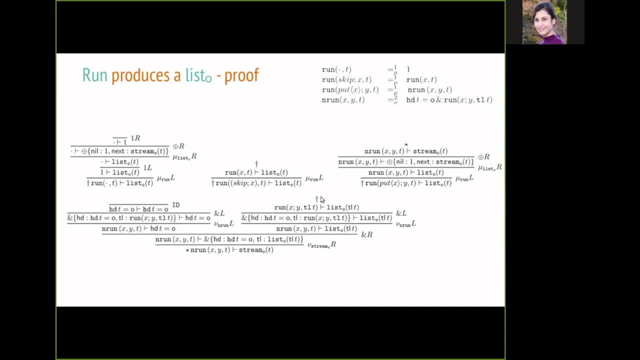 again the dagger judgment: um, so this path is only valid because we need to produce a list of this path, which is a fixed point, and we know that mu run here has a higher priority than new run, sorry, new n run. so, um, the two left, the two, the two fixed point left rules that we have on this. 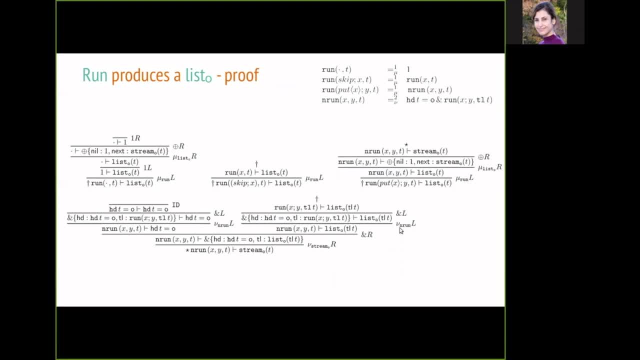 path. we know that um mu has higher priority than you, so we are good. if it wasn't the case, then we needed to find some right rule for you that has higher priority of um of other fixed-point rules applied on the right. Okay, so this is a valid proof. 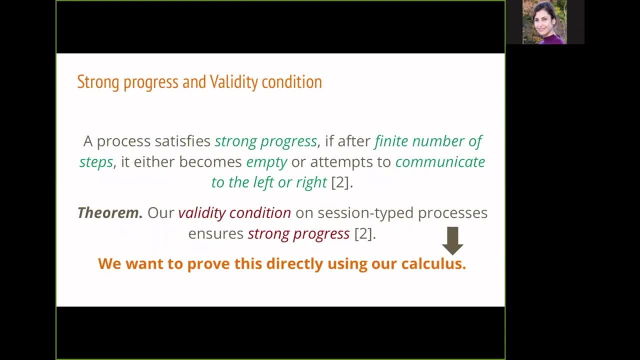 Okay, good. So up to here were a couple of examples. I introduced our calculus for simultaneous induction-coinduction and very briefly explained the validity condition that we need to check to ensure we have actual proofs and not just derivations. We also looked at an example of a program working on mutual listing rate as fixed-point just now. 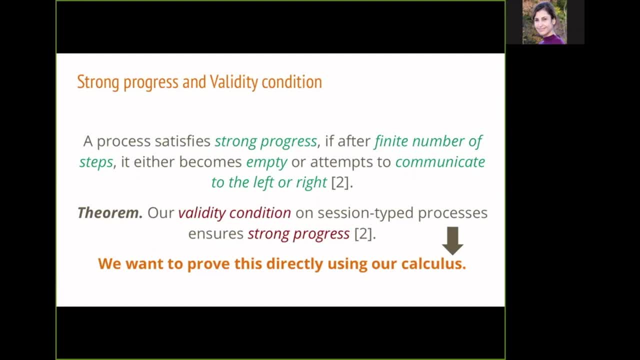 So all of our examples prove the property about some particular programs up to now, But we want to use our calculus to prove a more general result. Okay, so let's take a step back and talk about the third question we talked about earlier. What is the property corresponding to termination and productivity? 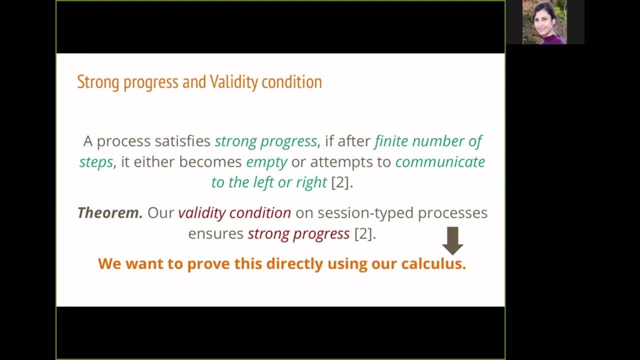 in a session-to-session type program that is defined over interleaved least and greatest fixed-points. The answer is a strong progress property. A process satisfies a strong progress if, after a finite number of steps, it either becomes empty or attempts to communicate to the left or right. 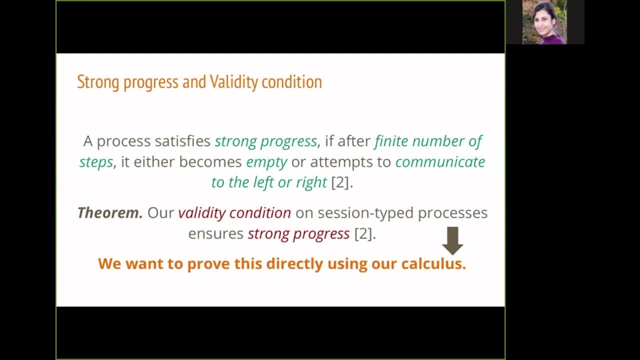 We have already proved that with a suitable local validity condition of processes that we introduced on session-type program, we can ensure the property of strong progress. Our proof is based on a Cori-Hovart correspondence between session types and linear logic. Now we want to use this calculus to prove our theorem directly. 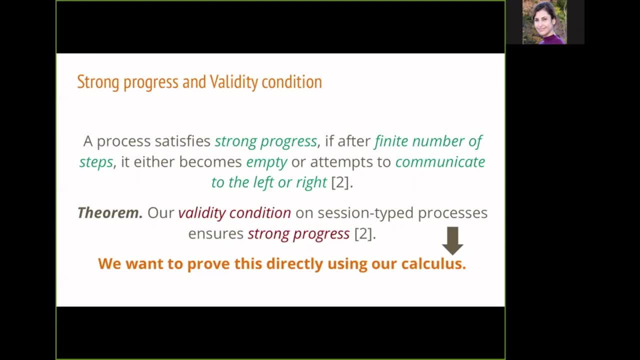 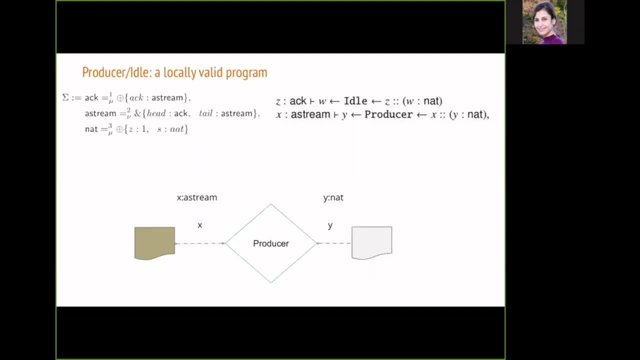 And the importance of this proof is that we may be able to use it to prove the same property for a more generalized local validity condition. To get a better sense of what a strong progress is, I put two animated examples of session-type processes in the slides. 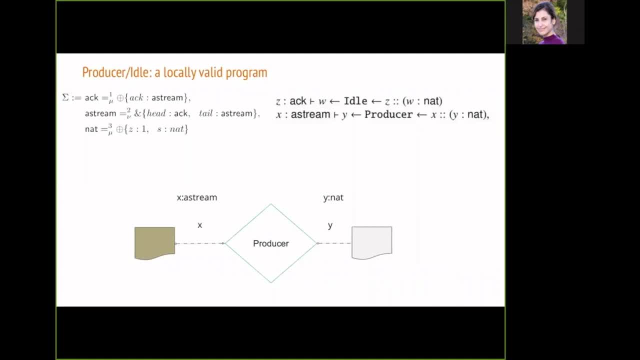 and here I focused on the higher-level description of them. If you want to see more details and their definition, you can take a look at the slides and also you can find them in our paper. So we have this process producer with two external channels: x and y. 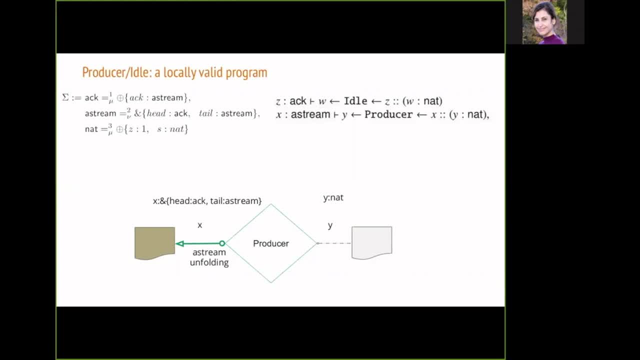 A producer first sends an A-stream unfolding message along channel X and then requests for the head from the process that offers along channel X. After that it goes into a new state, which we call it IDEL, and it waits for an acknowledgement along channel X When it receives the 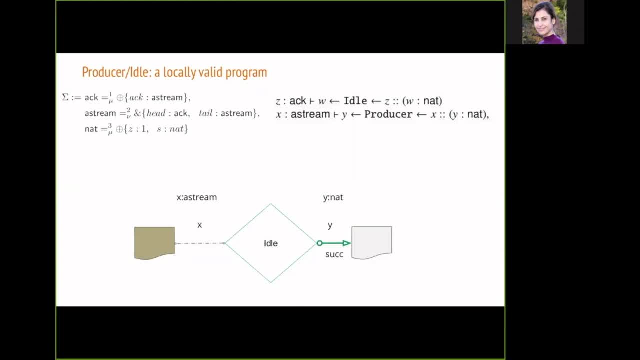 acknowledgement, it sends a successor as a natural number along channel Y and it goes back to the original configuration. So, as you see, in this loop producer actually communicated with its external channels X and Y. That is why we say that producer has this strong progress property And our local validity. 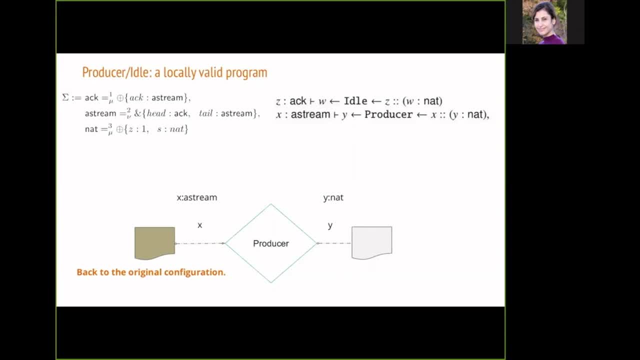 condition also accepts producer because it receives an unfolding response And the priority of this unfolding message is higher than the priority of the unfolding message that is sent along the same channel. As another example, let's look at PingPong, which is an invalid program that doesn't satisfy strong. 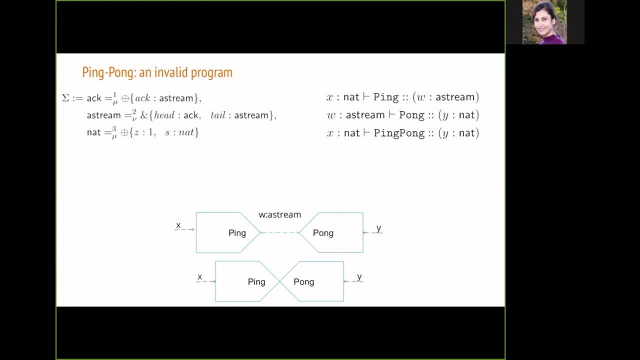 progress property. PingPong first responds as Ping and then continues as Punk. So PingPong sends an extreme unfolding message to Ping requests for head. Ping sends an acknowledgement to Punk And then we are back to the original configuration. So they loop forever. 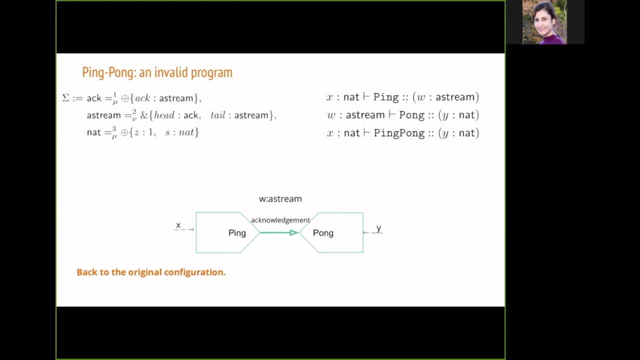 without ever communicating along channels X and Y. So as an outsider observer you will never see a trace of computation. you cannot differentiate ping-pong from a virtuous process. That is why we say that ping-pong doesn't have the strong progress property. But the fact is that. 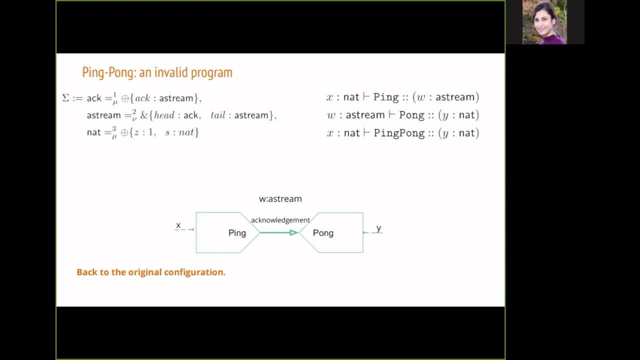 because of the halting problem, we cannot have an effective condition that captures all processes with some compositional strong progress property. So no matter how we generalize our condition, there are some processes that are missed out. But we want to generalize it as far as we can, The way that we. 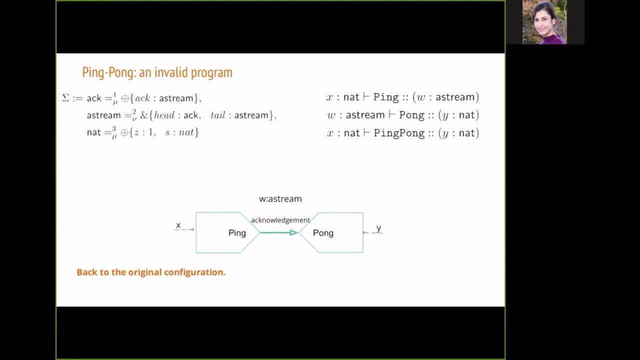 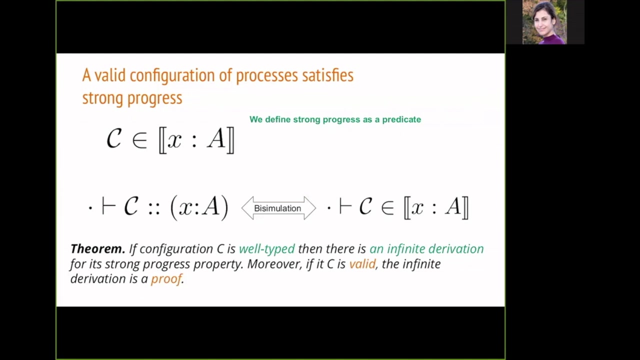 prove that our local validity condition implies a strong progress is by appealing to the validity condition introduced by Forty-Nine. So if you want to generalize this condition, we need a new alternative method for proving strong progress, And that is why we introduced our first-order calculus. In this setting, we can define a strong progress. 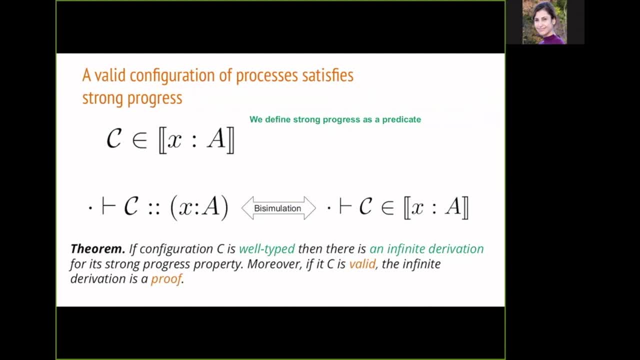 property as a predicate and we set it at a configuration that offers a long x has a strong progress if this predicate holds. Using a, by simulation we showed that the configuration type checks if, and only if, we have a derivation for this predicate and this derivation is a valid 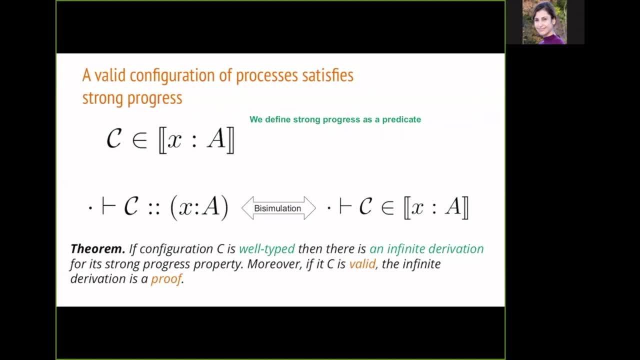 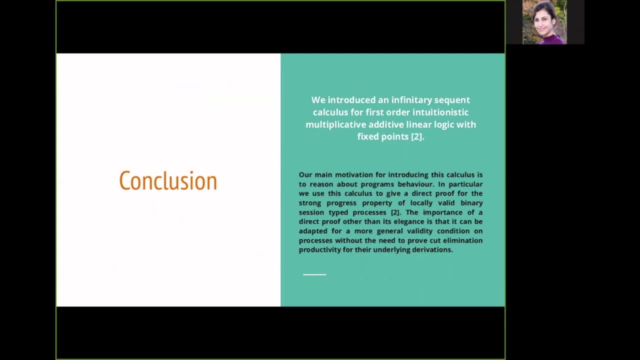 proof only if our configuration is locally valid. And this is a valid proof only if our configuration is locally valid. As a summary, we introduced an infinitely-sequent calculus for first-order intuitionistic, multiplicative, additive linear logic with fixed points, And our main motivation is to reason about program's behavior. In particular, we want 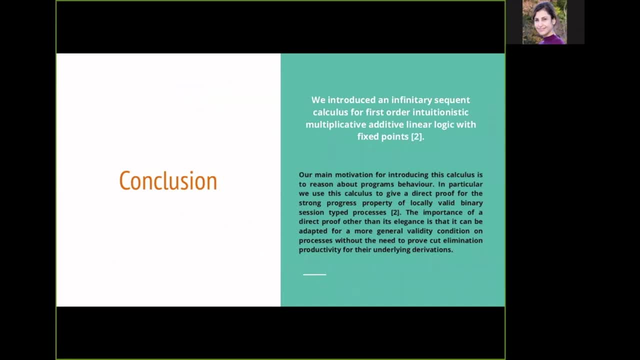 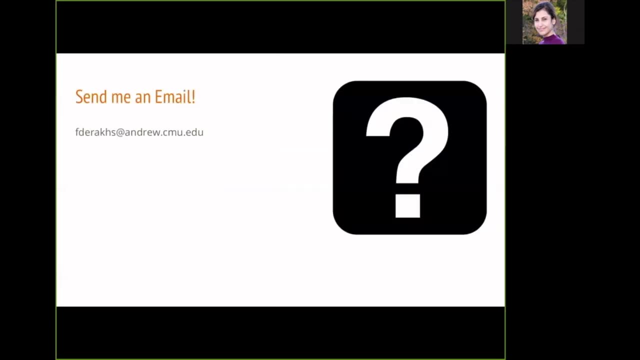 to use this calculus to give a direct proof for the strong progress property of locally valid binary session-type processes. Thank you for your attention And if you have any questions, comments or suggestions, please send me an email.